Now I had to pose this on thefel and tell, as there are two subconscious points in this work piece. There are tube- krót miał and tube- assistir, so these are performance measures of whole division of the material at the bottom. The other two is the wandering act Age. of the material is explained by every teacher in the math lab. Here we have two kitchen gin- değişät 이걸in Waldo Braille siewar and a wrapped screw- the string. although this is a gross, the track of material is thick after removing it. what is that? that? 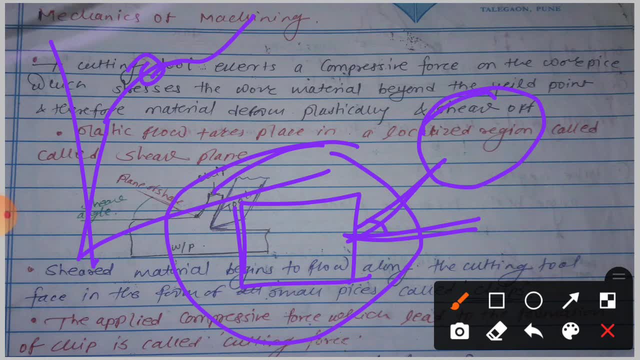 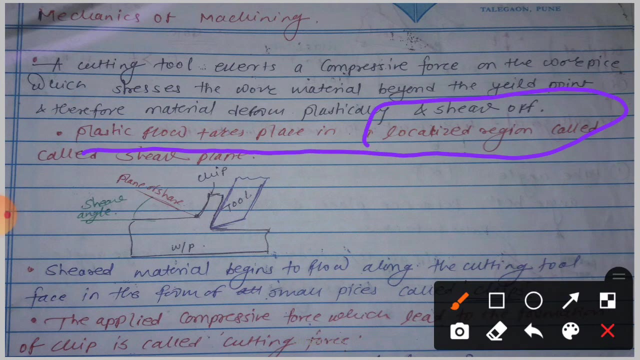 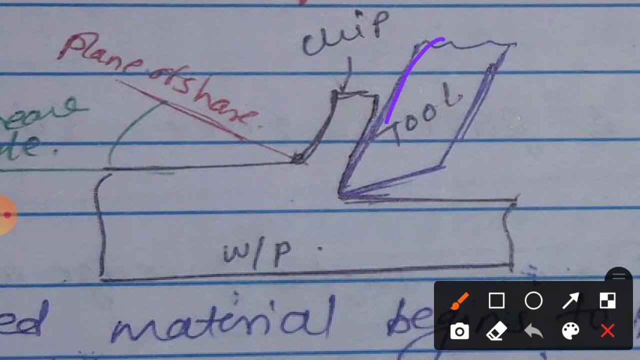 which is supposed to you is a. For example, a form of a create can be made from a. The plastic flow takes place in a localized region, is called as the shear plane. The cutting tool is applying force on the work piece and the force generates the compressive stresses in the work piece. 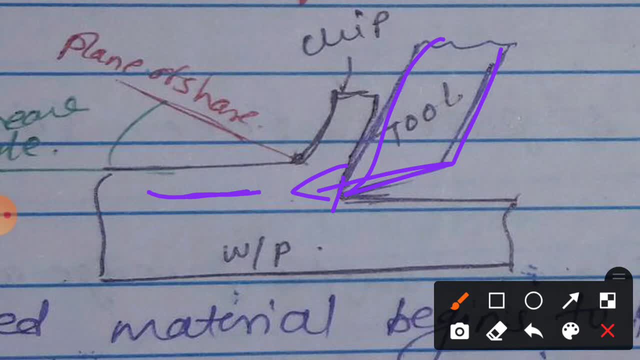 And due to the excessive stress of the work piece material, the upper layer of the work piece is being removed And the shear of the location is being removed From this location. the material of the work piece is being shear off to this location. 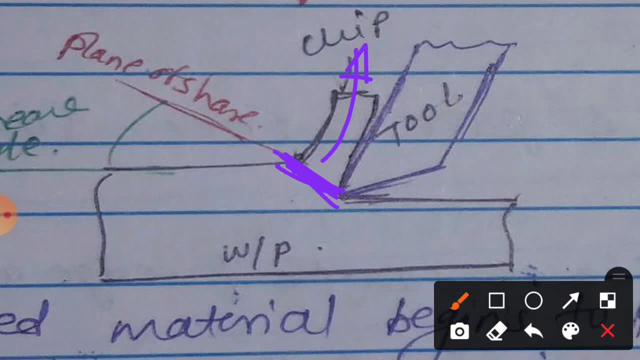 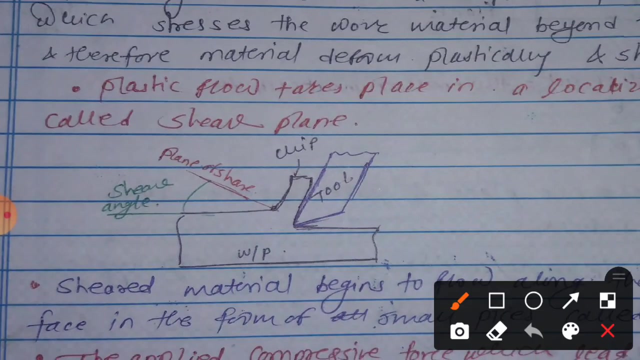 In this location the shear plane is called as shear plane And the material that is being removed from the work piece, the material that is being removed and the flow is happening on the face of the tool, is called as shear plane. Shared material begins to flow. 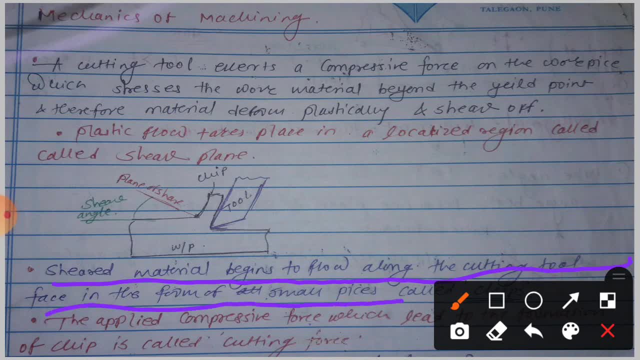 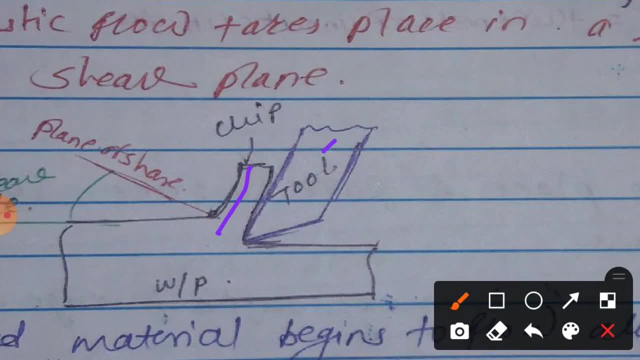 Along the cutting tool face in the form of the small piece is called as the chips, The material that is being shear off, that is being removed, and along the tool face, the material that is being shear off and along the tool face. 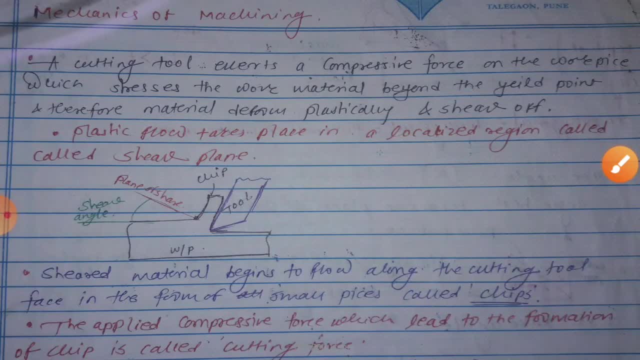 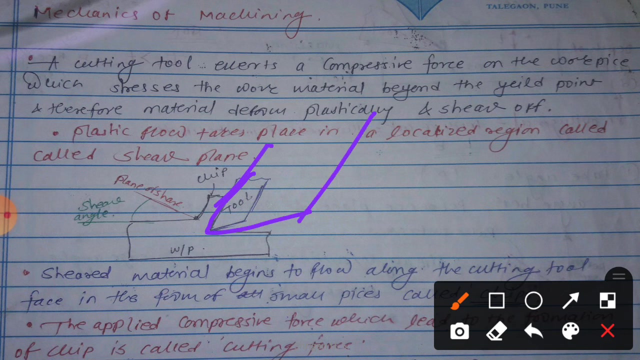 the material that is being shear off is called as the shear plane. The applied compressive force which leads to leads to leads to formation of chips, is called as the cutting force. That means that, because of the compressive force, the function of the tool is 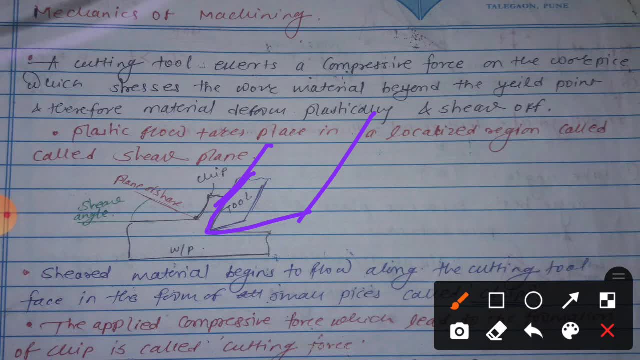 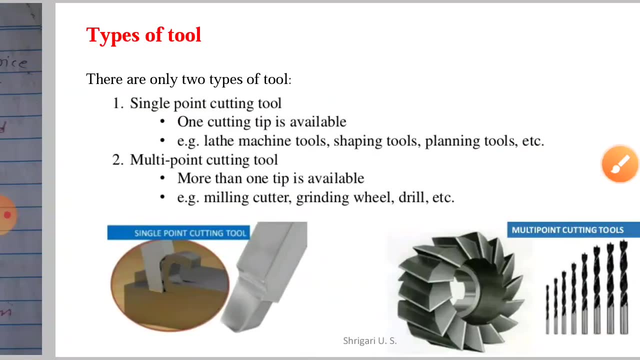 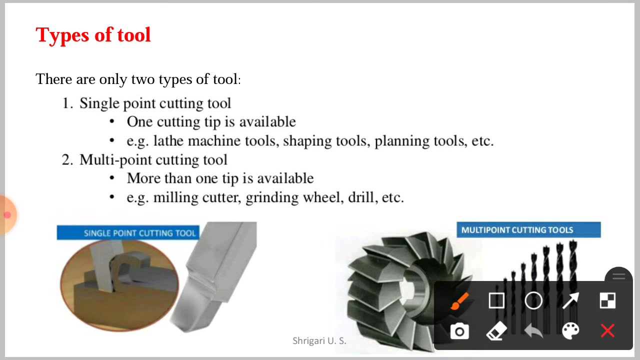 making it realized in the process of work piece. in the process of work piece, if the material is shear off or chip is being removed in that condition, In that condition we call it as cutting force. Next point is of tools. There are mainly two types of tools. 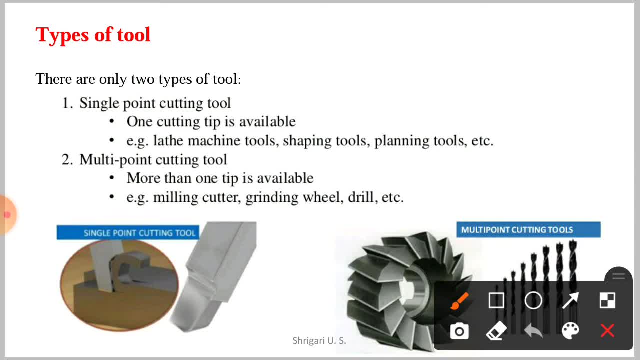 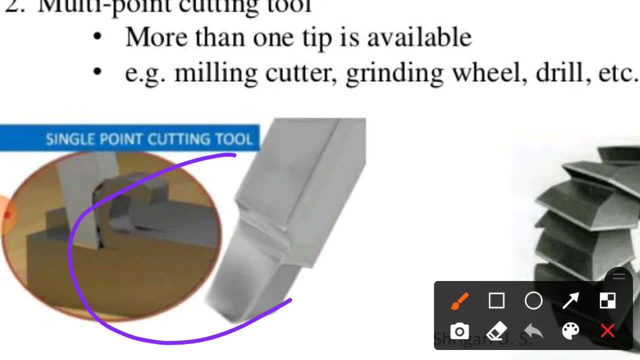 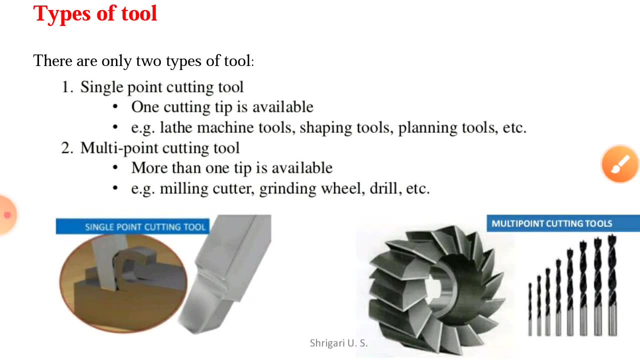 First is single point cutting tool. one cutting tip is available means in single point cutting tool there is only one cutting tip and if you see lathe machine, shaper machine or our planing machine, in that single point cutting tool, single point cutting tool, is used. 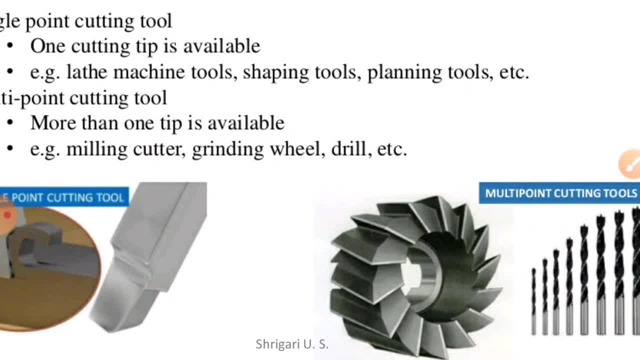 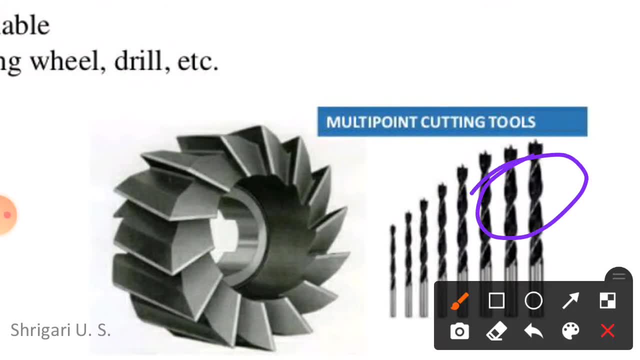 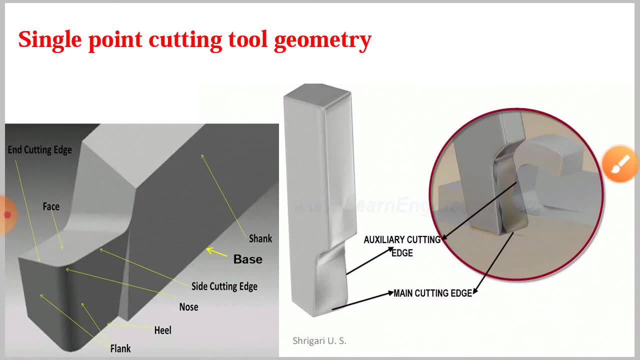 and in multi point cutting tool more than one tip cutting tip is available. if you see milling cutter or drilling cutter in that number of tips are available cutting tips. it is called multi point cutting tool. next is single point cutting tool geometry. single point cutting tool geometry. if you see here: 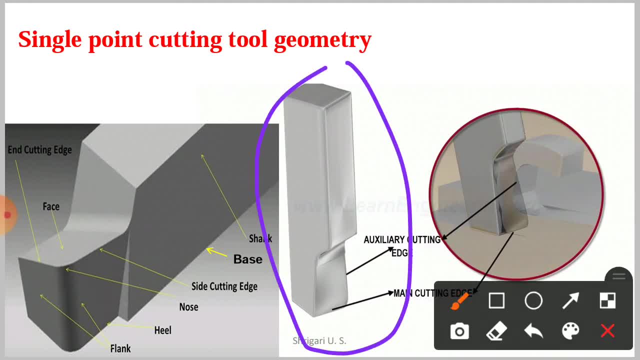 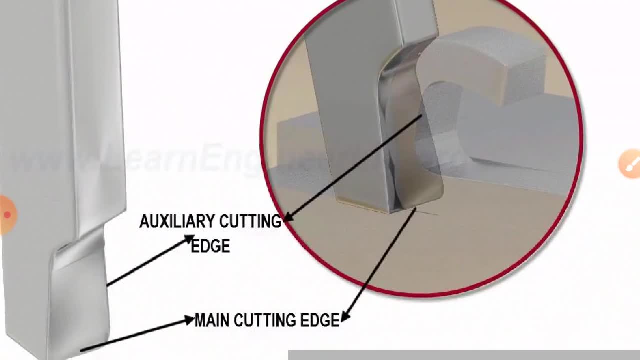 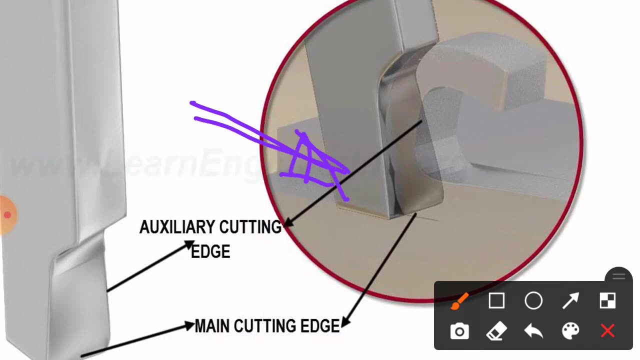 in 3D cutting tool is shown here. if you see this cutting tool when it moves against work piece means when it moves against work piece, then compressive force. that compressive force is applied in tool, so material starts to shear off and that material shear off from two edges. 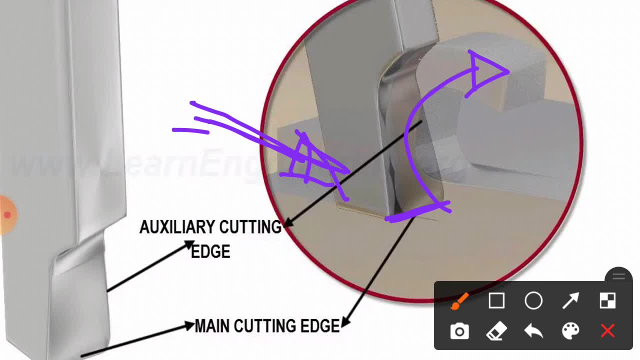 first edge is this A edge of tool, material is removed from here. and second, if you see, if you see here work piece surface finishing is done, material is removed from here means this surface material is removed from this. edge means this tool has two cutting edges. one is main cutting edge and 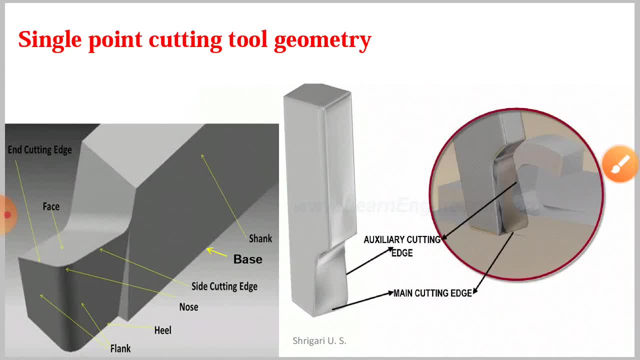 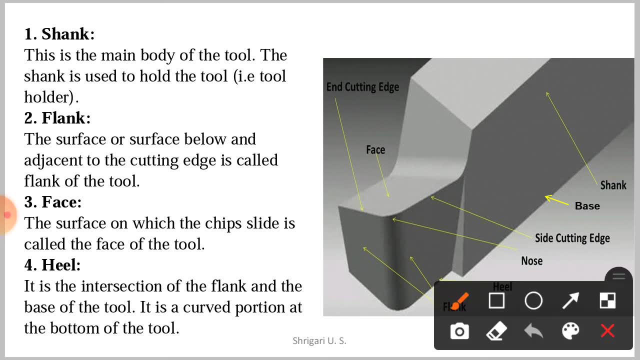 second is side cutting edge. next is we have seen deep measure tool geometry. first point is shank. shank is the main body of the tool. the shank is used to hold the tool means the tool in tool post, in the portion where we hold the tool. 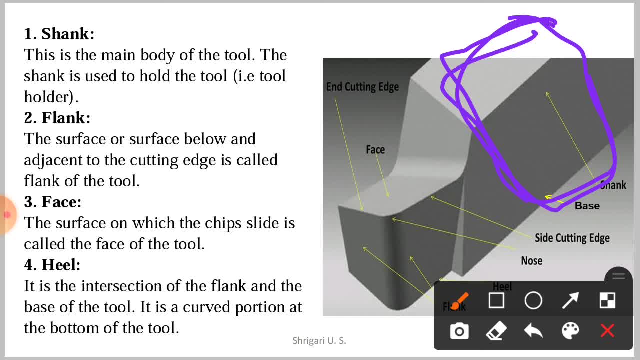 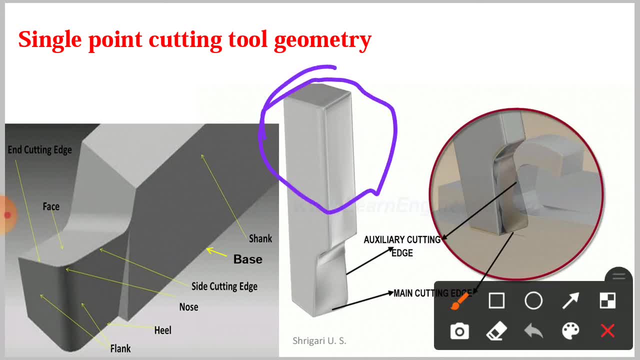 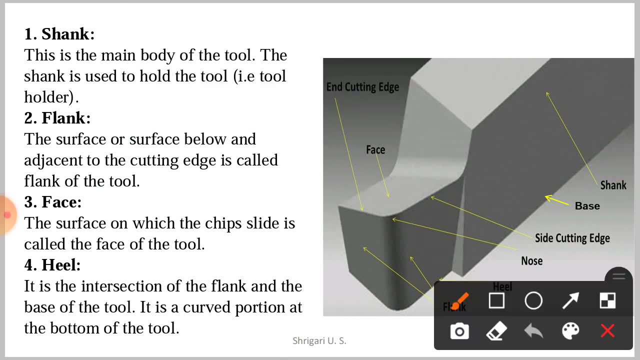 the portion where we hold the tool that is called shank. you know that this tool, this portion, is called shank. next is next is flank. the surface, or the surface below and adjacent to the cutting edge is called the flank of the tool. means the surface which is just below the cutting edge. 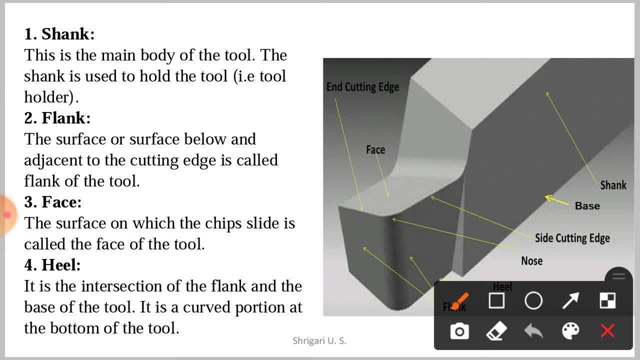 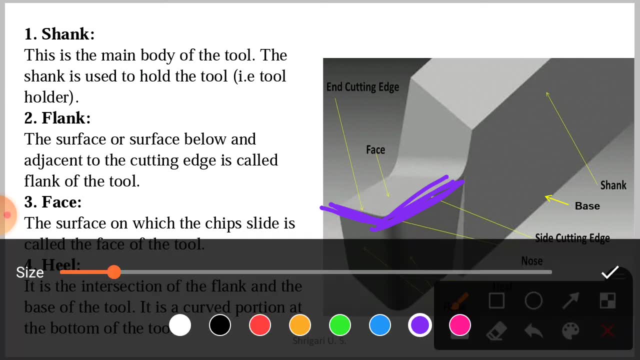 it is called flank. so if, if you see this tool, I told you that there are two cutting edges- one is main cutting edge and second is side cutting edge- then just below the side cutting edge, just below adjacent surface, if you see this surface, this side cutting edge, 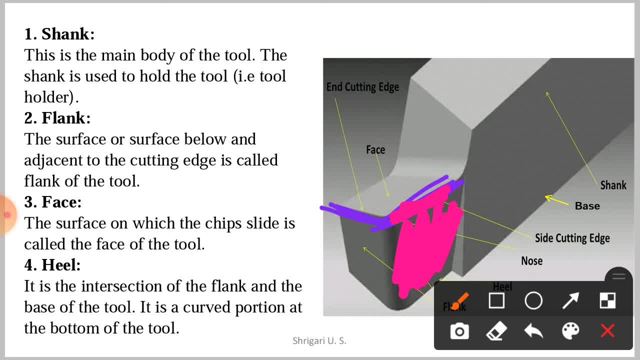 just below, just below, just below surface side cutting edge, it is called flank side cutting edge, flank. and if you see again that this edge, this is the main cutting edge, its below surface, just adjacent and adjacent to the cutting edge and below surface, it is called flank. next is face. 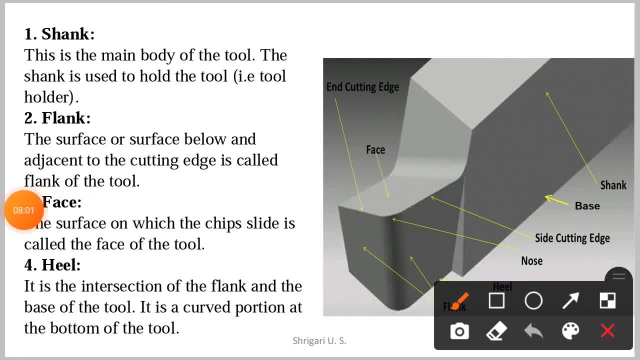 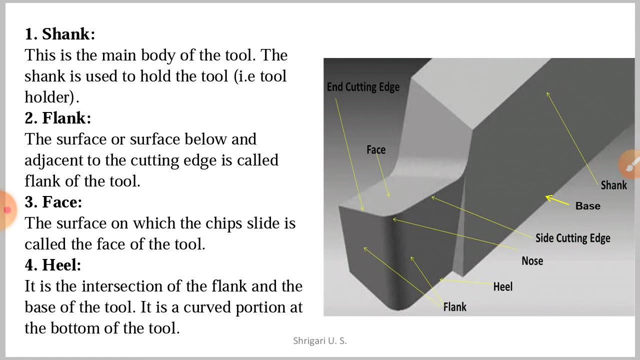 the surface on which chip slides is called, as the face means on which chip slides, on which chip slides, it is called face. if you see this surface, chip is erasing. if you see previous slide, if you see this slide, in this slide, the chip is erasing. 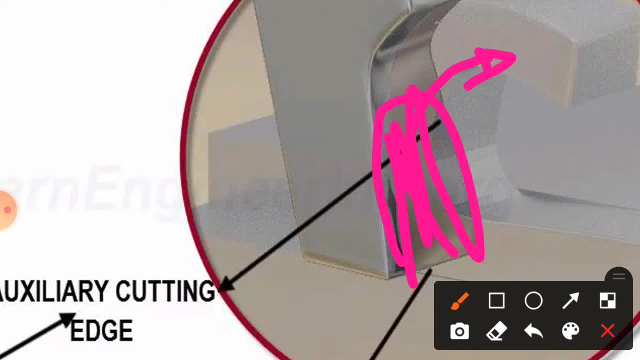 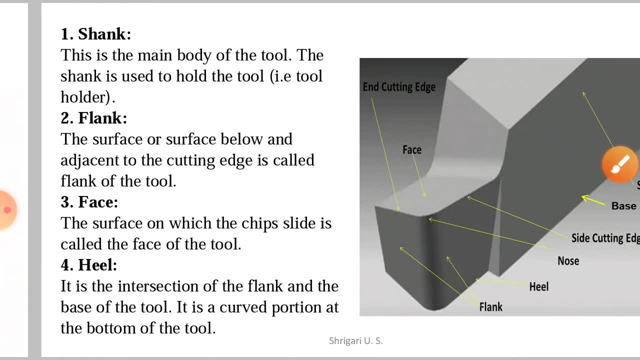 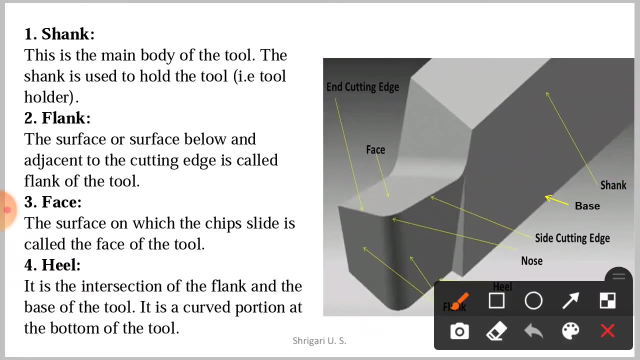 and from which surface it is sliding these surface. they are sliding on this surface. this is called face. next is hill. what is mean by hill? It is the intersection of the flank and the base of the tool, Means the base of the tool and the flank. This intersection is called as heel. 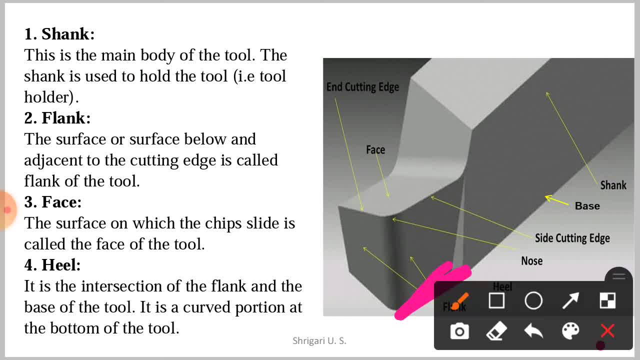 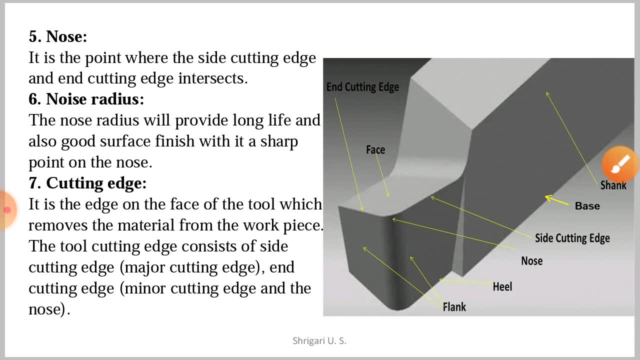 Means. this is the session and this is the heel And this is mainly curved shape Means. it is provided a small radius In the bottom side. Next point is nodes. What is mean by nodes? It is the point where It is the point where slide cutting edge, Side cutting edge and end cutting edge are intersects. 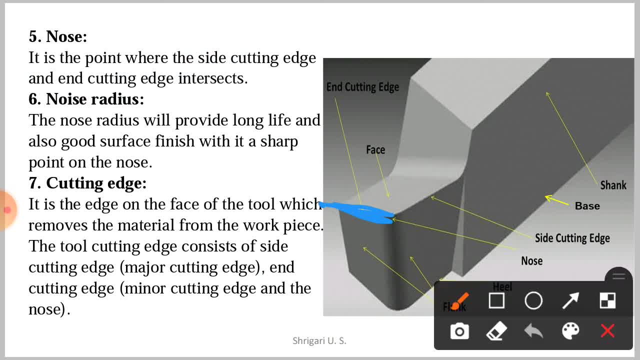 Means: end cutting edge and side cutting edge. Where ever they intersect, They are intersected. Now side cutting edge and main cutting edge are intersected. Next point is nose radius. Nose radius will be provided to long life of the tool And for a good surface finish Means. this nose is provided a small radius from the edge corner. 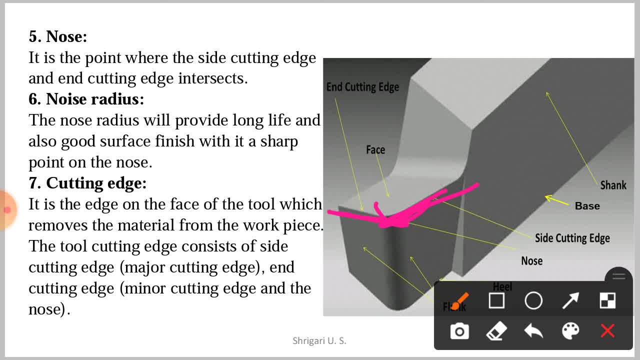 Because of this, the life of the tool is increased And surface finishing of the tool is good. Next point is cutting edge. Cutting edge means It is the One minute. It is the edge on the face. It is the edge on the face of the tool Which remove the material from the work piece. 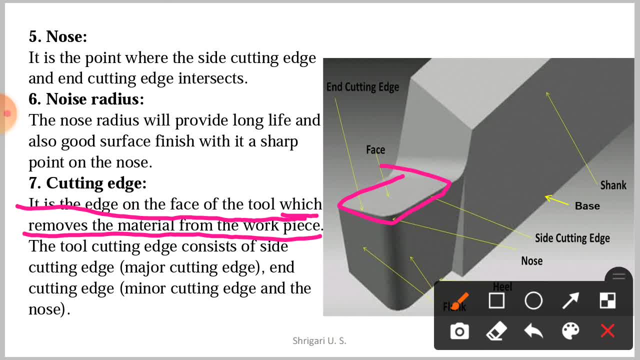 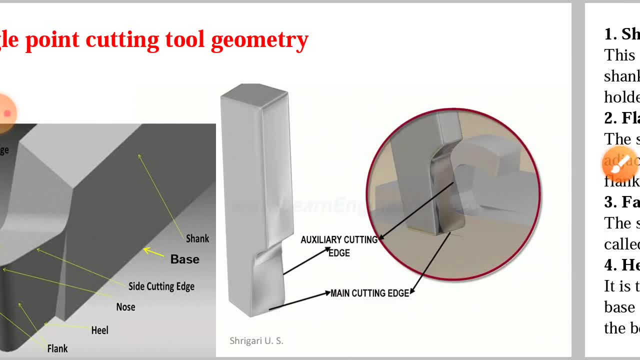 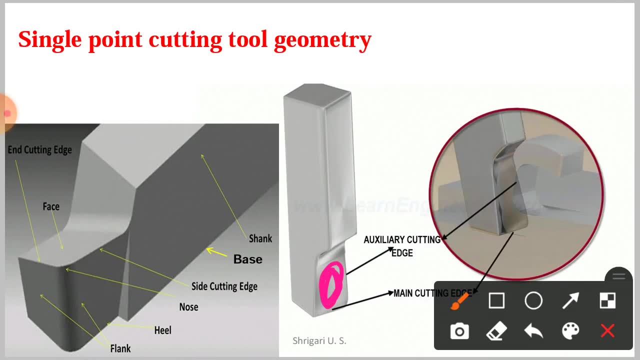 The face, The edge on the face Which remove the material from the work piece. That is called cutting edge. If you have seen the previous slide, I told you that Which face, It has two edges. That is why it removes the material. One is this edge and the other is this edge. 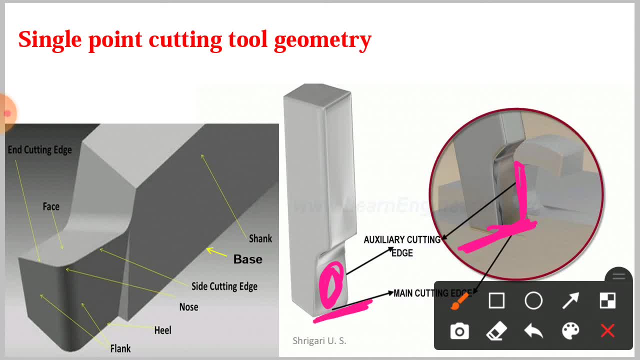 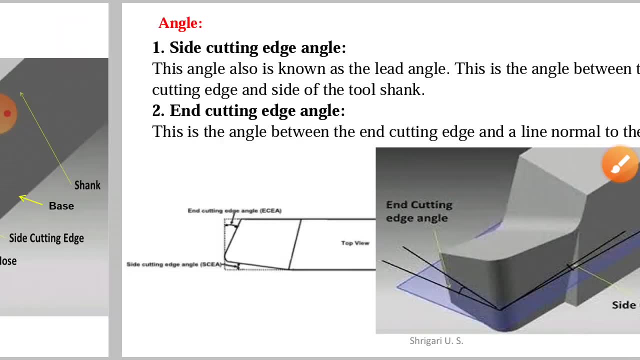 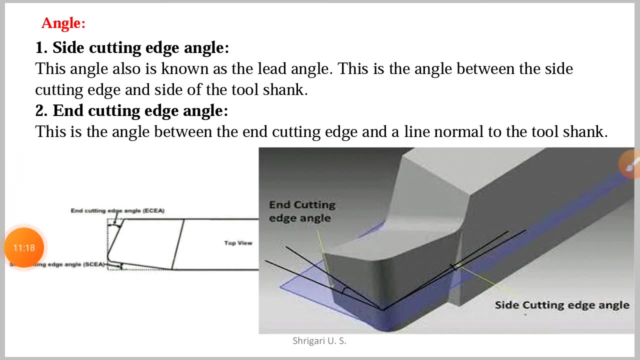 So this edge, This edge is called main cutting edge And this edge is called side cutting edge, One minute. Next point is angles Angles. First angle is side cutting edge angle- Side cutting edge angle. Next is side cutting edge angle- Side cutting edge angle. This is the angle also known as the lead angle. 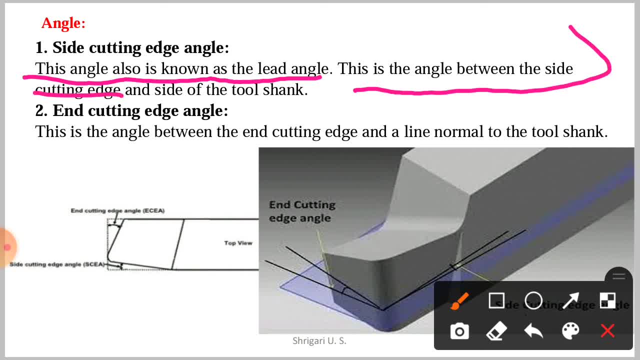 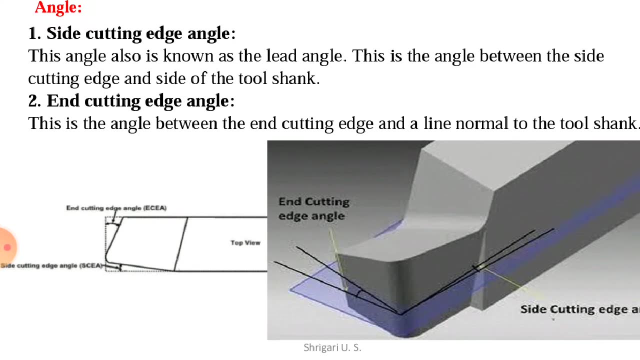 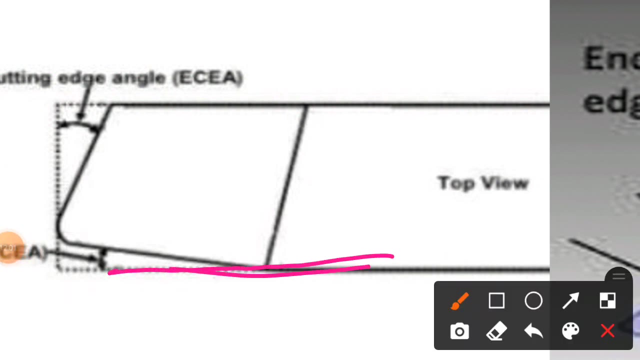 this is the angle between the side cutting edge and the side of tool shank. means the angle between the side cutting edge and the side of tool shank is called as side cutting edge angle. you can easily understand in this figure: the angle between the side cutting edge and the side of tool shank is called as side cutting edge angle. 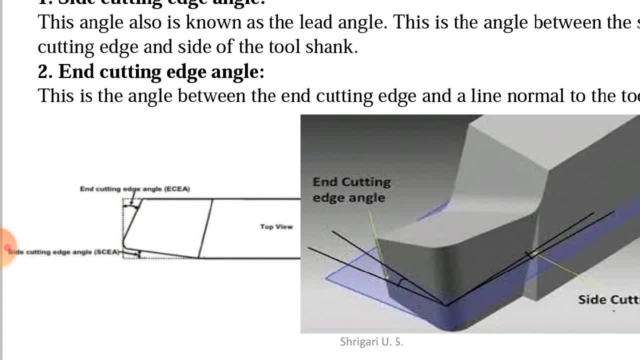 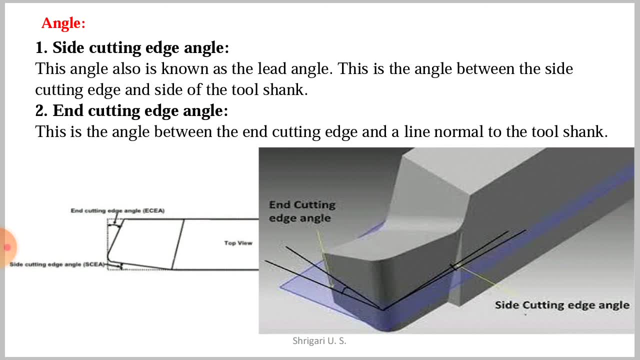 and this is shown on the top view of tool shank. you can easily understand in this figure. you can easily understand in this figure: or we can measure this angle on the plane which is parallel to the base means we can measure the plane which is parallel to the base. 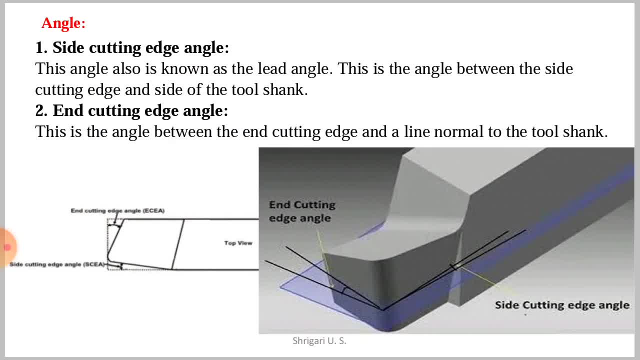 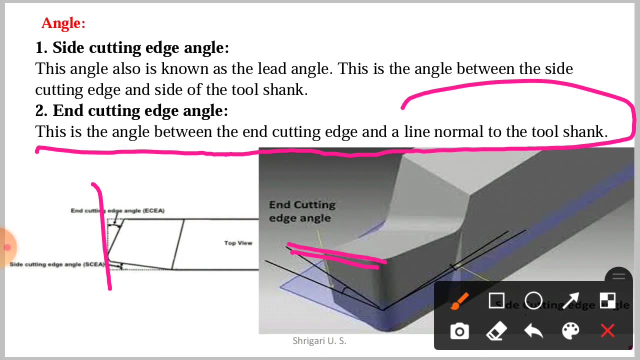 next time. end cutting edge angle. this is the angle between the end cutting edge and the line normal to tool shank. means the end cutting edge. means the end cutting edge. this is the angle between the side cutting edge and the side of tool shank. this is the angle between the side cutting edge and the line normal to the plane which is parallel to the base. 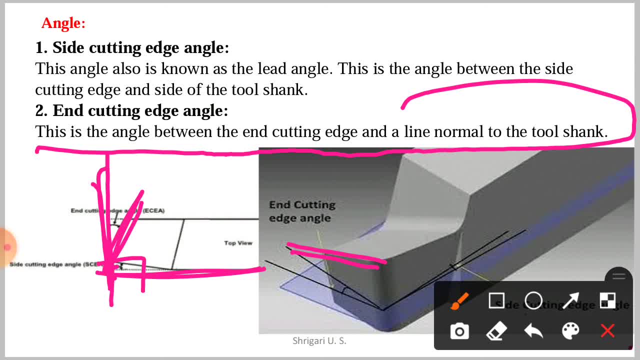 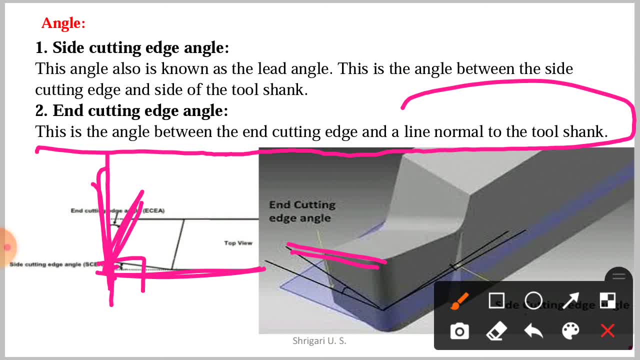 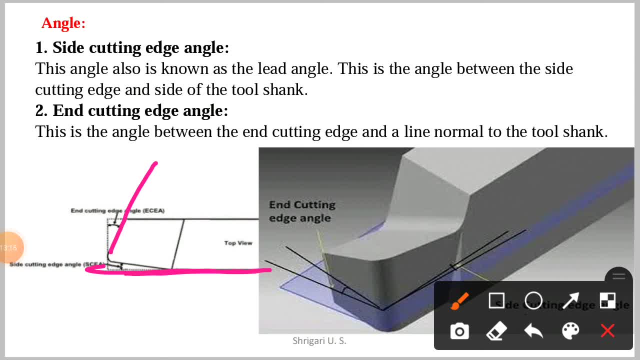 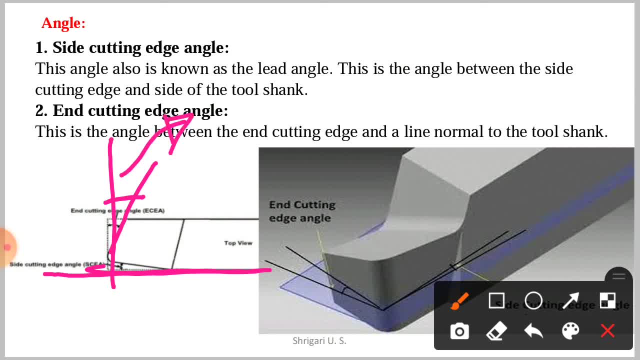 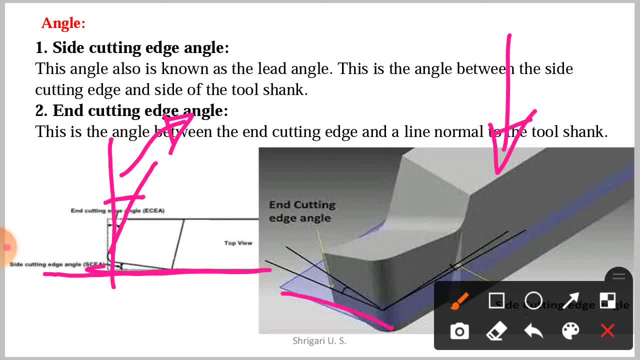 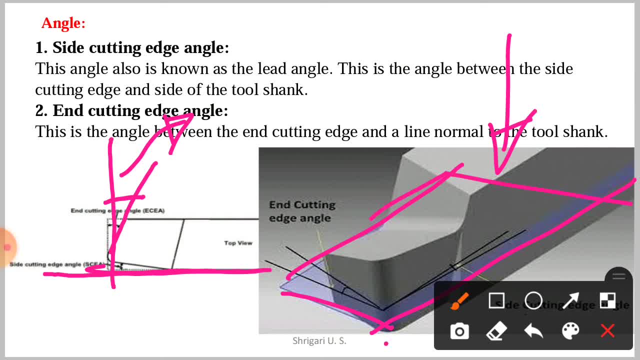 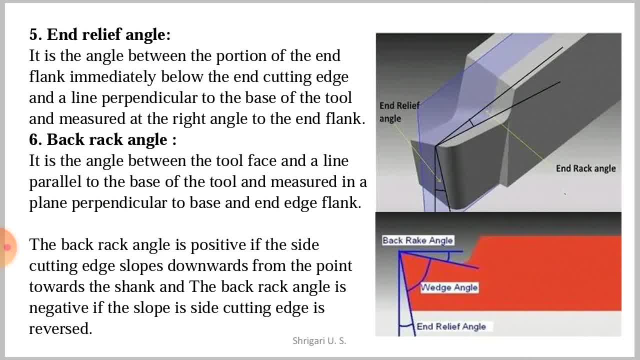 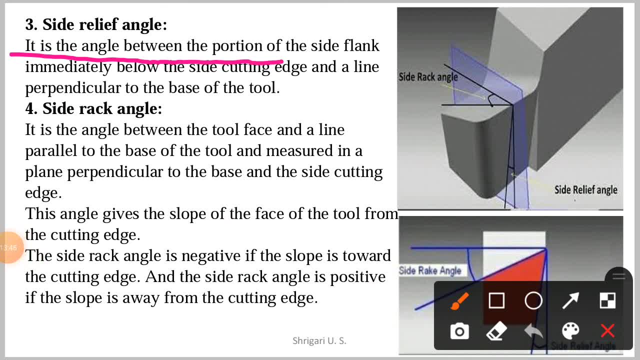 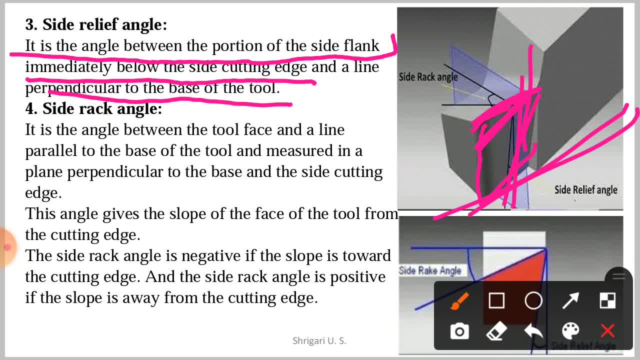 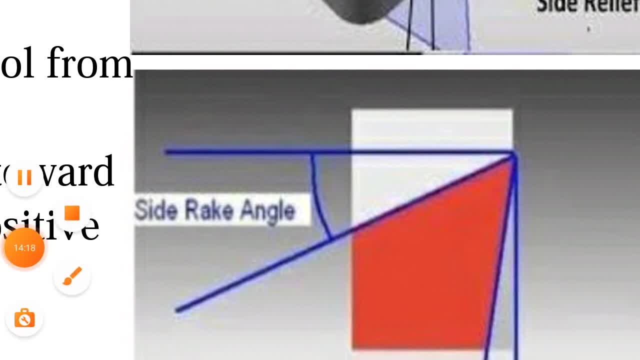 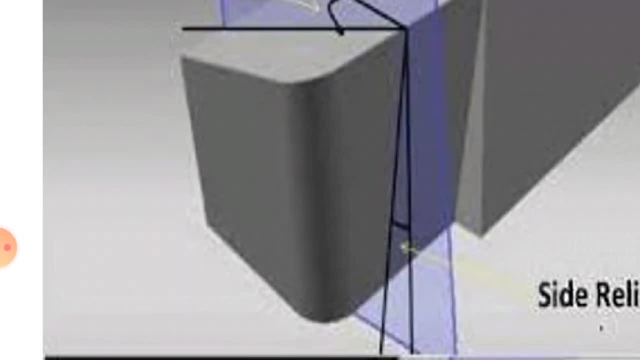 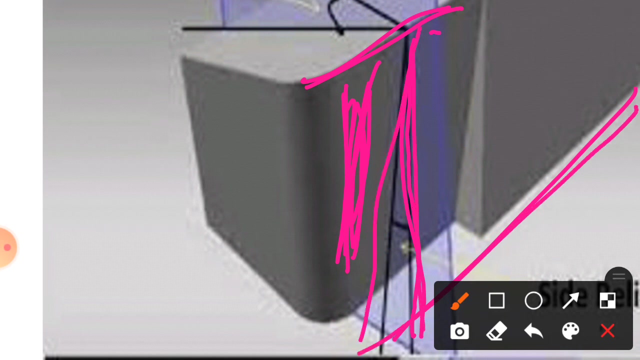 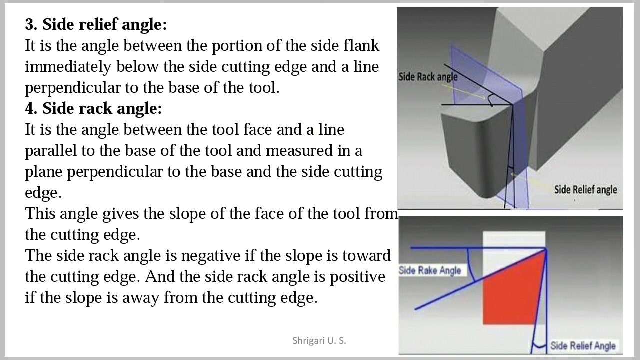 This is the side cutting edge of the below flank and this is the normal to the base. This is the line and this is the normal to the base. These two angles are called as side grip angle. Next, side grip angle: It is the angle between the tool face and the line parallel to the base of the tool. 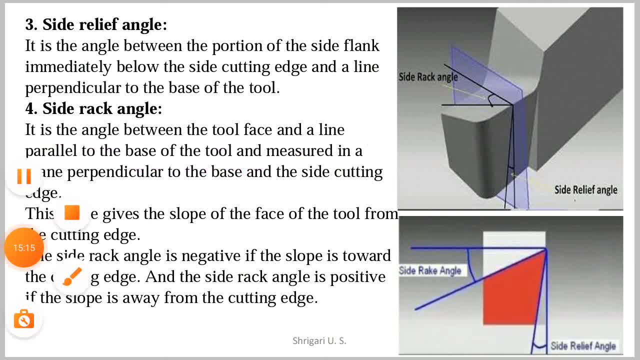 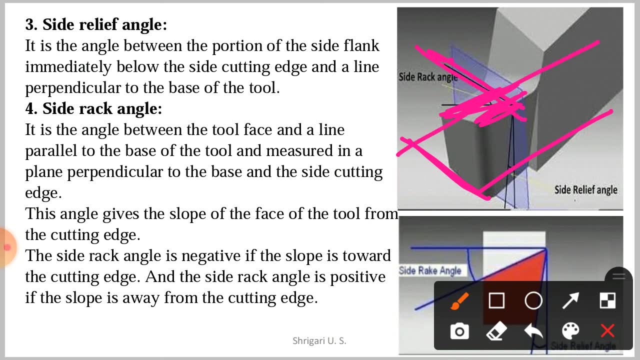 Means the face of the tool and the line which is parallel to the base. The base has parallel line. This- two lines are angles- means this is the angle between the two sides. side-grip angle means you have seen that parallel to the base. 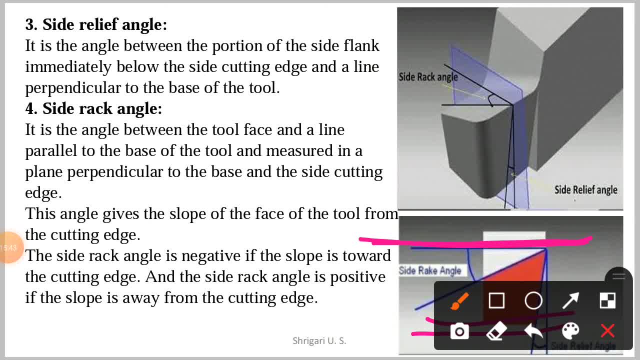 parallel to the base is this line and the face of the tool. this is the side-grip angle and these two angles- side-grip angle and side-grip angle- if we want to measure on some plane, it is measured on the plane which is perpendicular to the base. 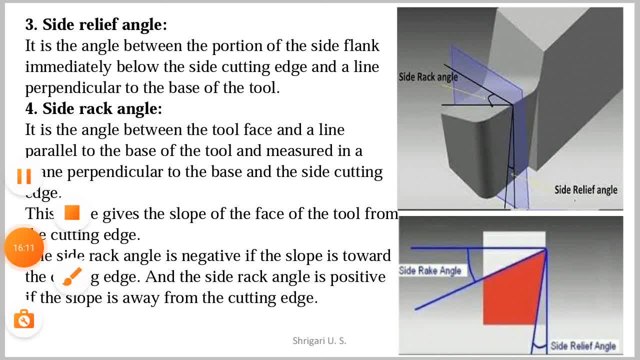 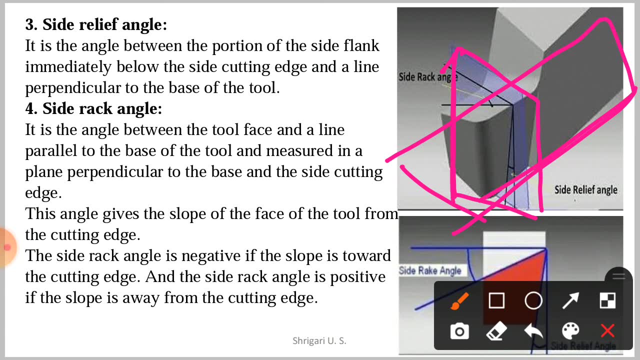 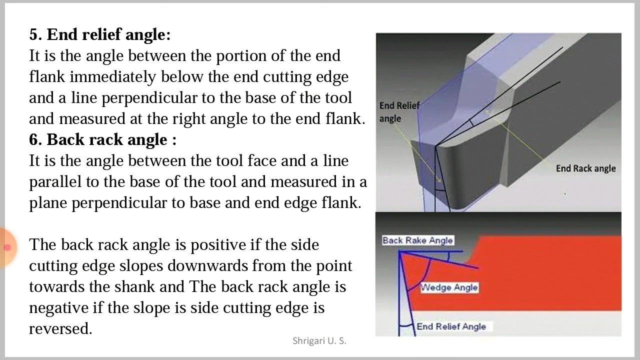 and perpendicular to the side-edge angle. these two angles are moving on the plane. if the plane is perpendicular to the base, then the plane is perpendicular to the base, then the plane is perpendicular to the side-edge angle, and these two angles are moving on the plane. next is end-grip angle. 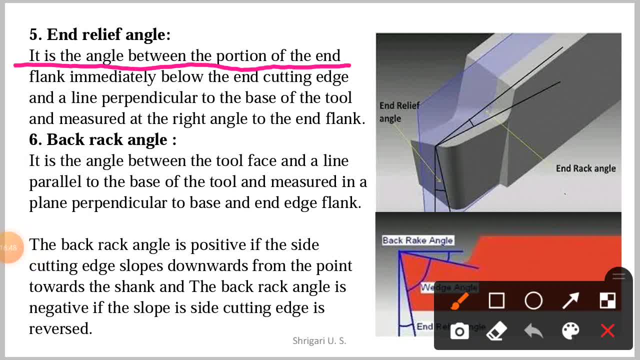 it is the angle between the portion of the end flank immediately below the end-cutting edge and the line perpendicular to the base of the tool means it is the angle between the portion of the end plank immediately below the end-cutting edge. the angle of the end-cutting edge is just below the plank. 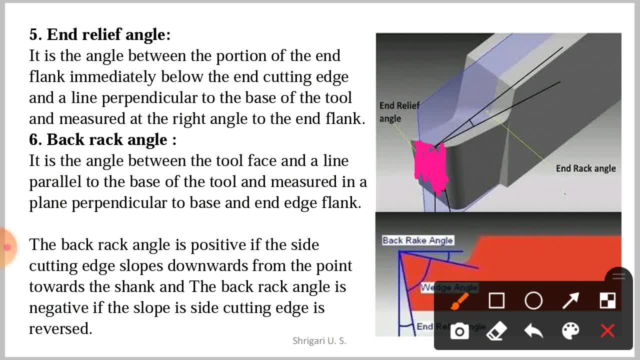 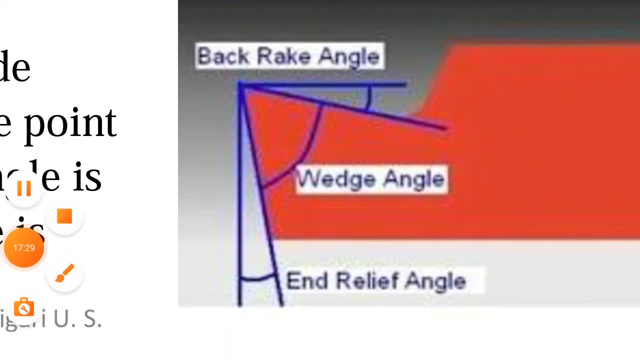 means just below the surface. and if you measure on the plane which is perpendicular to the base, then the angle between the two is called as end-grip angle. I will show you in this figure. as you can see, the base has a perpendicular line and the end-cutting edge is just below the flank. 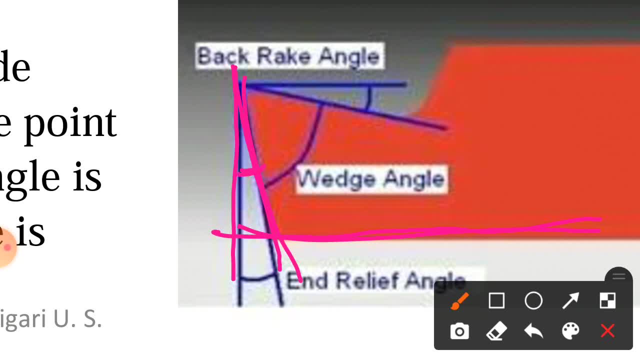 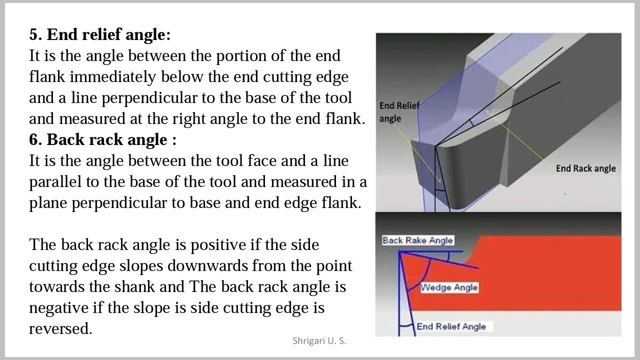 so the angle between the two is called as end-relief angle. next is back-grip angle. it is the angle between the tool face and the line parallel to the base base of the tool, means the tool face, this is the tool face, this tool face and the base of the tool.